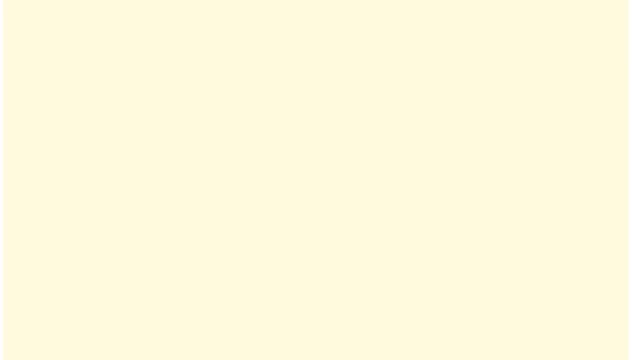 So I'm sort of going to go through the way which you're probably going to be learning when you learn how to do these, and it's a nice logical way to understand what's happening when we increase a number by a percentage. But then I'm going to show you a couple of shortcuts you can use to increase a number by a percentage or decrease a number by a percentage. 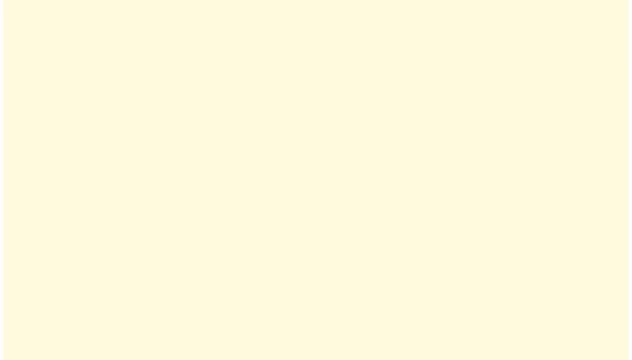 So I'll give you an example of the type of question we get with this. So say, I wanted to say I had the number 50 and I want to increase it by 20%. So I want to increase 50 by 20%. 20, by the way, 20% here, you might remember, is just a number out of 100. 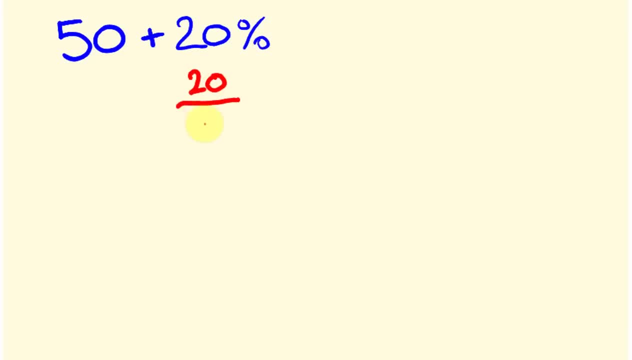 So 20% literally means 20 out of 100. Okay, So if we could work out what 20% of 50 was. this is the first way. I'll show you how to do it. then I'll show you the other ways. my third way: 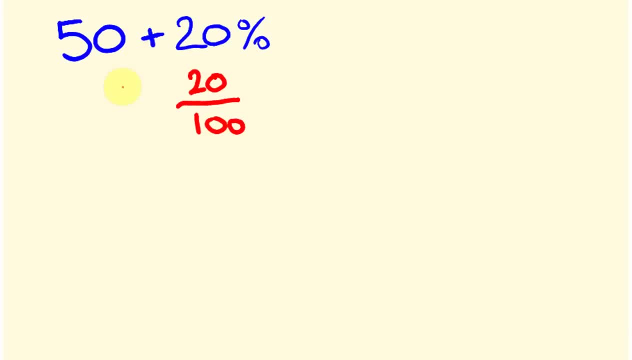 If you could work out what 20% of 50 was, you could add it to 50, okay, So you'd work out what 20% is and then you'd add it to 50 and you'd find out what 50 plus 20% is. okay. 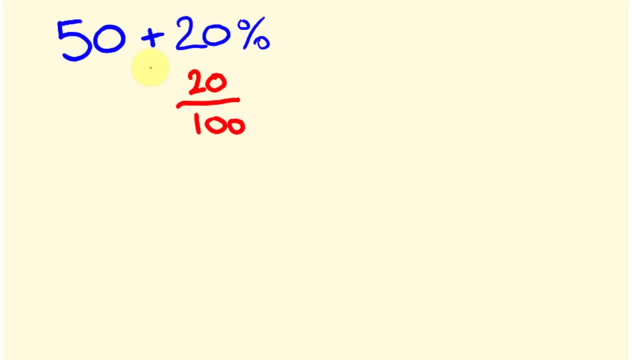 Where you increase it by 20%. So let's work out 20% of 50.. So we use this fraction form of 20% here, 20 over 100.. And we to do this, we times it by 50, okay. 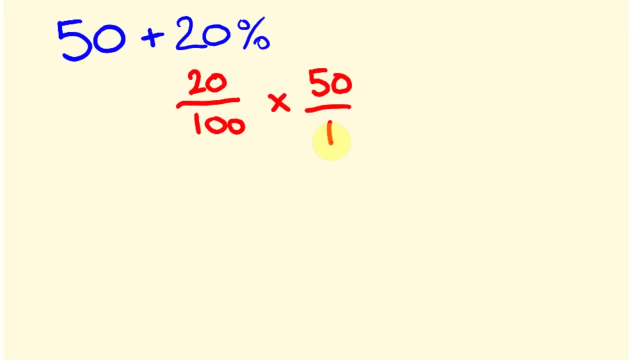 So 50 over 1, okay, And if you're not sure how to do this, I have some other videos that do look at this, okay. So what we now can do, as you might remember, is you can start cancelling our numbers, okay. 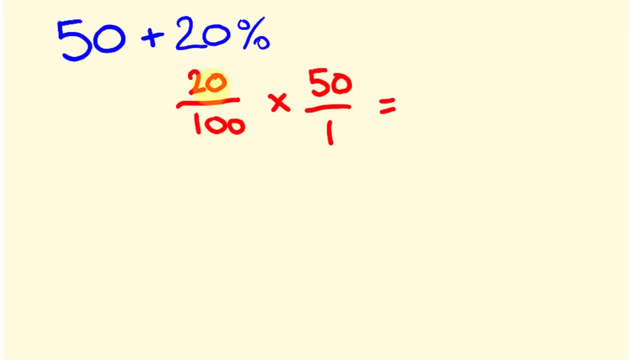 You can start dividing the same number into the top and the bottom, So 10 goes into both- this number here and this number here- so we can get rid of those zeros. 10 also goes into this number here and this number here, so we can get rid of these zeros. 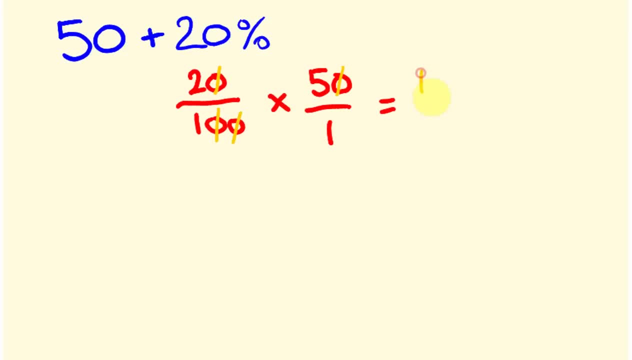 And what we're left with is this: 2 times 5 is 10.. 1 times 1 is 1., And this equals 10.. Okay, so what now I'm going to have is this: I'm going to have 50, and I'm going to be adding this 20% of 50 to it. 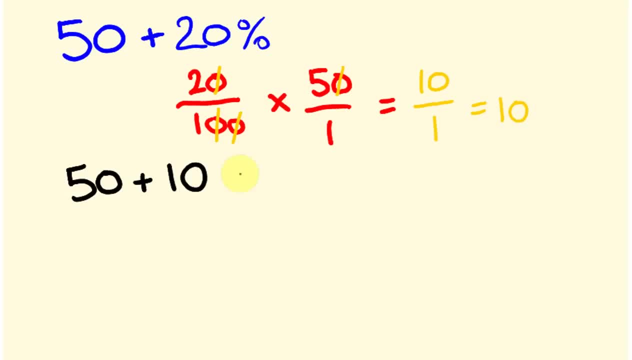 So I'm increasing it. 20% of 50 was 10.. So 50 plus 10 equals 60,. okay, That's a way that you can really really easily work out. you know how to increase, say 50.. 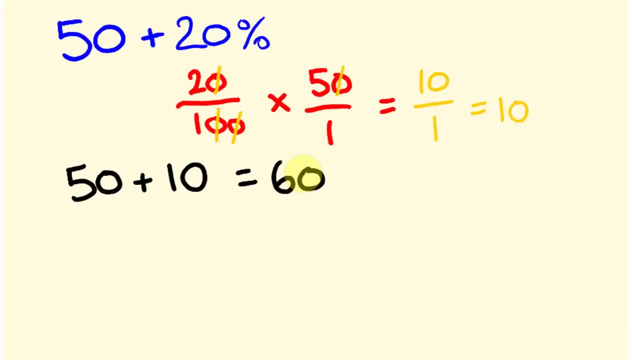 By 20%, okay, Or whatever number, by whatever percent. Work out what the percentage of it is and then add it on or decrease it if you're trying to decrease by a percentage. But I'll show you a little shortcut that you can use with this. 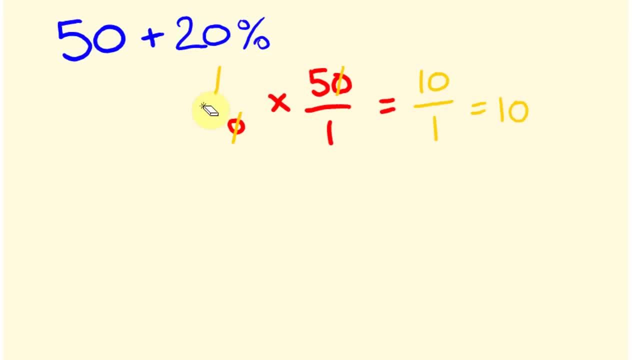 And this is as follows: okay, So you might want to keep that answer in your head as 60,. okay, Because we'll use that same sort of problem And I'm going to try and explain this now where you might. it's just a little conceptual thing here. 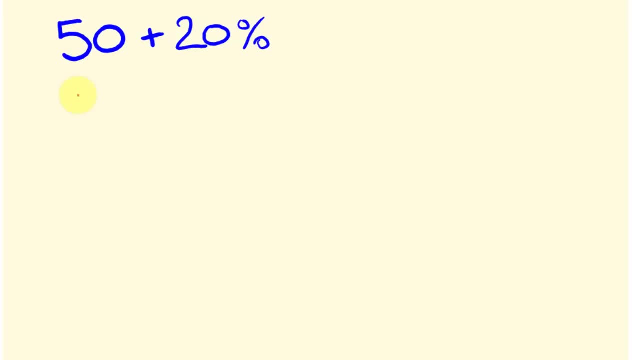 a little idea that might help you understand this, If you can understand that we're starting. We're starting with this whole amount here, this 50, okay, I'm going to just draw it as a circle here. It's almost like a 1, okay. 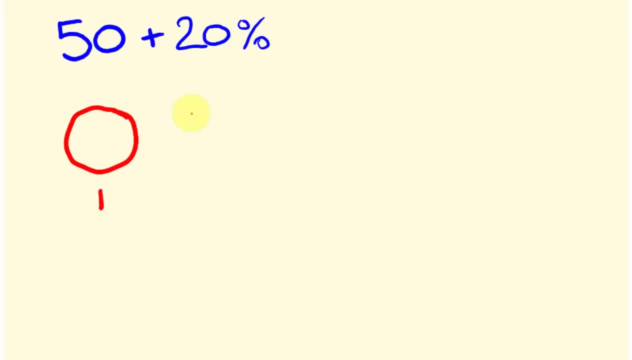 It's the whole thing, but it's worth 50,. okay, And I'm going to, I'm trying to increase this by 20% of this amount. okay, Which the other thing you might understand of this: this is not only 20 out of 100,. 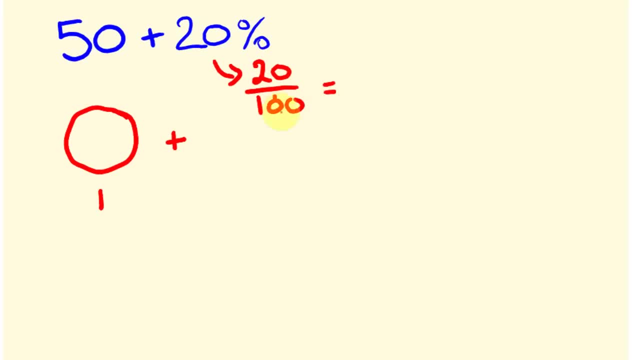 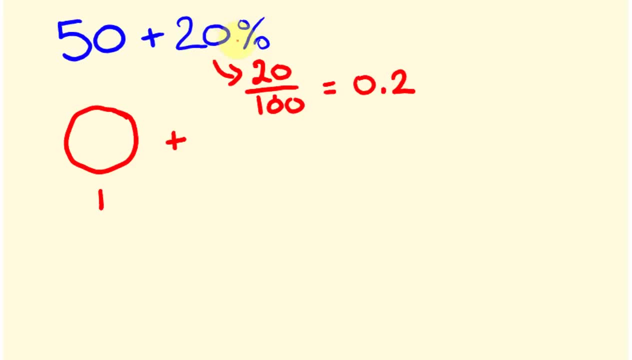 Okay, Another way you can work out. you can convert from a percentage to a decimal really quick- is just divide this number by 100, move the decimal place twice 1,, 2, and you get 0.2.. So we have the decimal form now of 20%. okay, 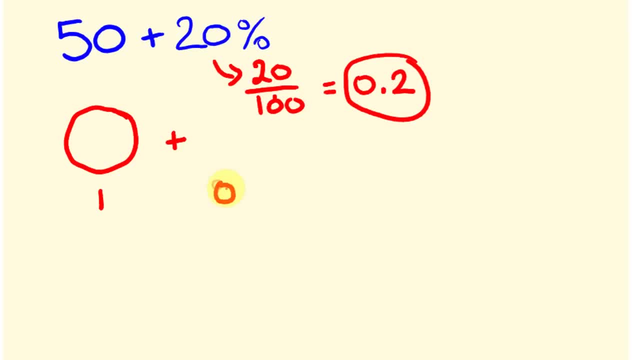 So I want to increase it by 0.2, okay. So really, what I'm doing is I'm actually trying to find out what 1.2, okay, So I've got the 1 here and I'm adding 0.2 to it. 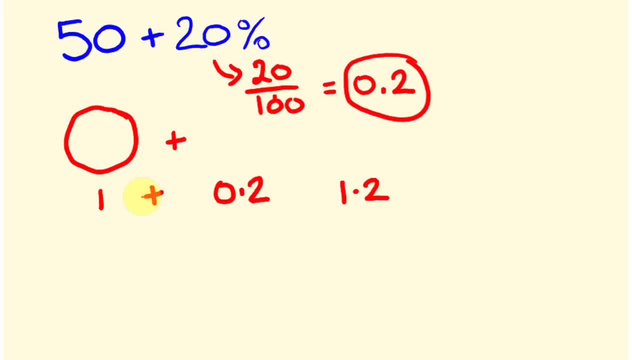 1.2,. okay, So I'm going to add these together of 50 years. okay, So 1.2 times 50. Okay, Do you see this? Hopefully I'll go through a few examples in a little bit. 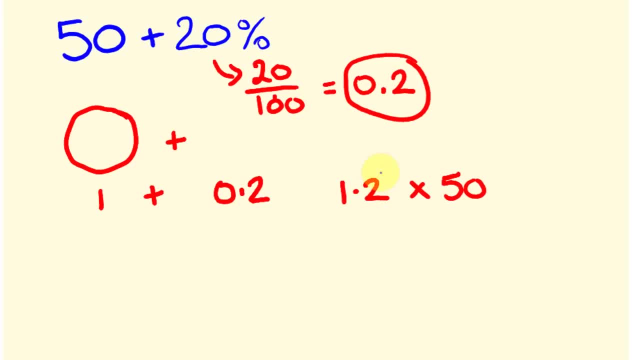 So 1.2 times 50, this is very much the same as 12 times 5.. 12 times 5 is 60.. Okay, All right, I'll give you an example of again how you might actually convert these sort of things, okay. 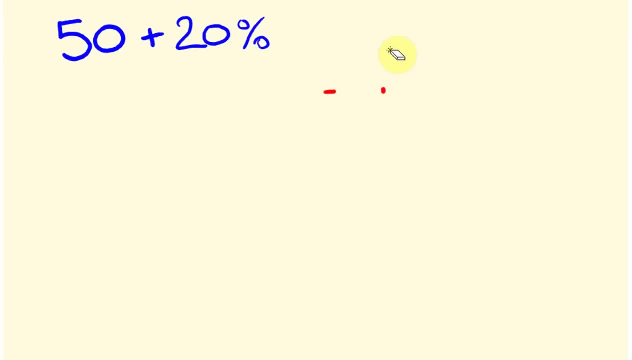 So I think I may lose a few people with that. They go: what's going on there? And so I'll try to re-explain this again. I'll try to give you a few examples of what you would get say with some questions. 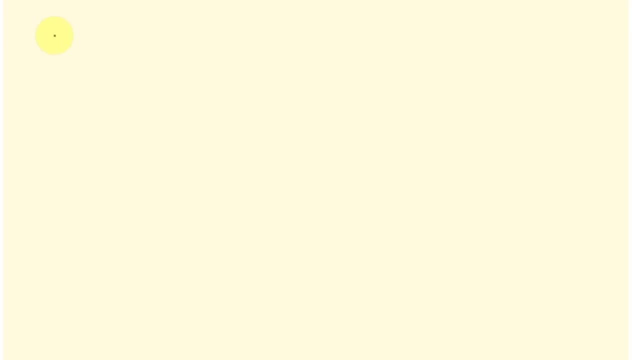 Say we were trying to- not even where I'm working them out straight away, but where I'll just show you the equation you would be doing to work it out. So say we wanted to work out what We had- 70, and I wanted to increase this by 30%. 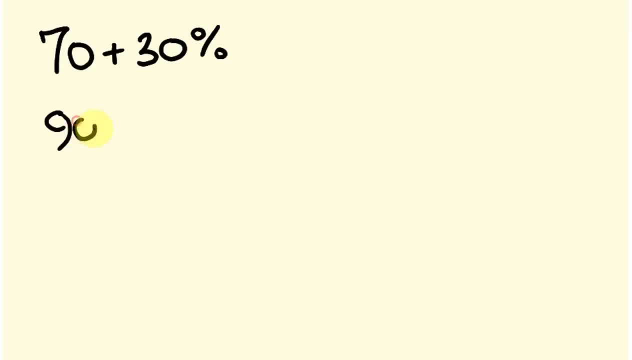 Or I had 90, and I wanted to decrease this, Or I had 100, and I wanted to increase this by, say, 12%. Okay, So there's a couple of questions here. Now, the way that you would set this up is as follows. 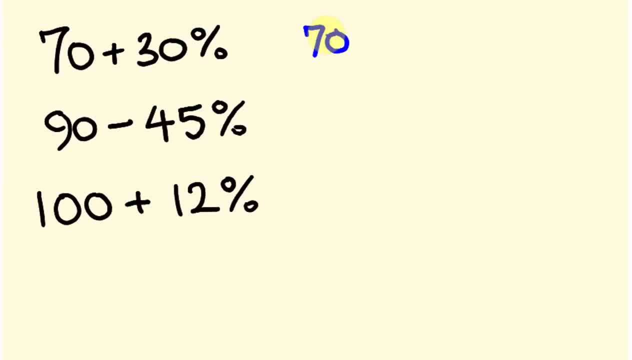 It's the same as getting 70 here And this is going to be a 0.3.. So this is the one part, but this is a decimal is 0.3. So I add this because I'm adding it onto this. 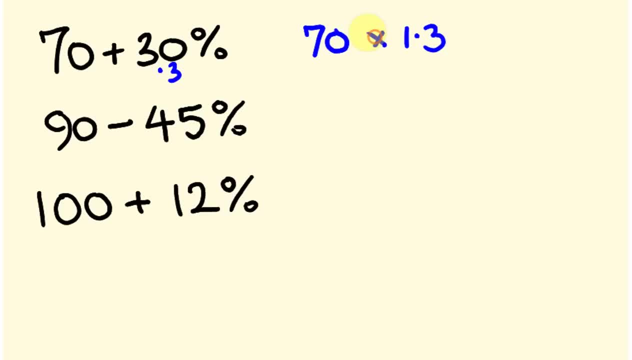 This part. here. I've got 1.3, and I'm timesing these numbers And that will give me my answer. Okay, So you might be able to work out what that is. That would be 91. Okay. 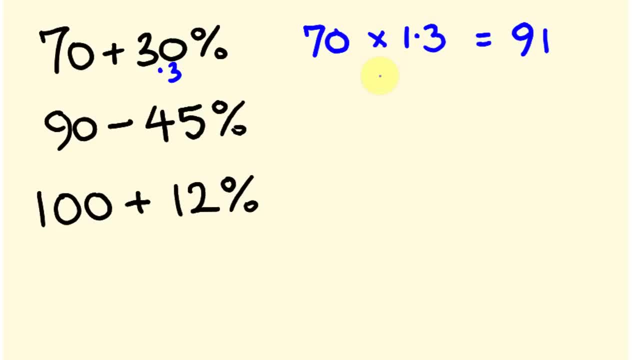 Because 7, 3's are 21,, plus 70 is 91. What about we do say I wanted to take 45% off? You might see the trick with this one, Because this again, as a decimal, is 0.45.. 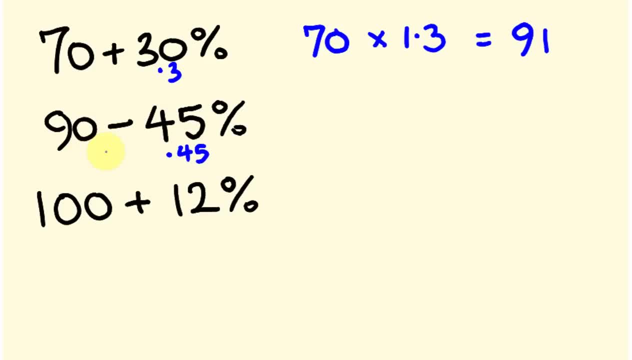 But now I'm not adding it to this one part Here. I'm taking it away. Okay, Because this one we had 1, and we're adding it to 0.3.. This one, we're taking it away. 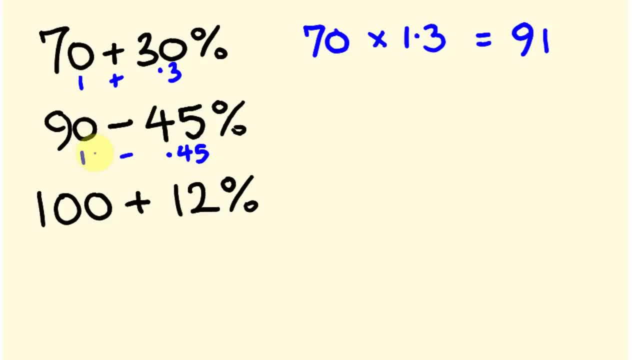 So what we're actually ending up with is 1, take away 0.45, is 0.55.. Okay, And I'm going to be timesing this by 90.. Okay, So what's the answer to that? 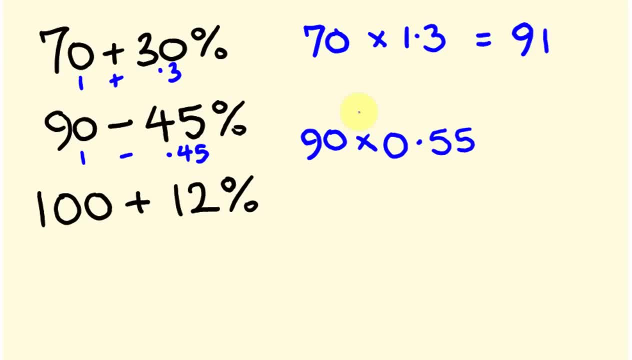 Well, The way that you might work this out is as follows. I mean, you could just times these guys straight out, But I would try to think of this, maybe like this, If you could imagine this: 0.5 here, which is half of 90,, which is 45..